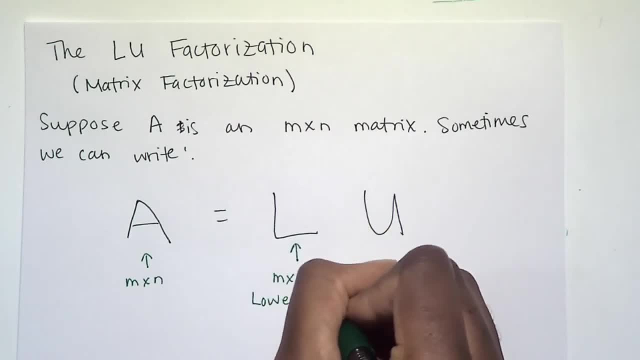 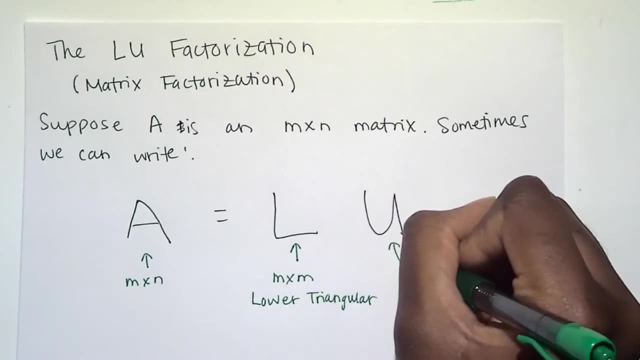 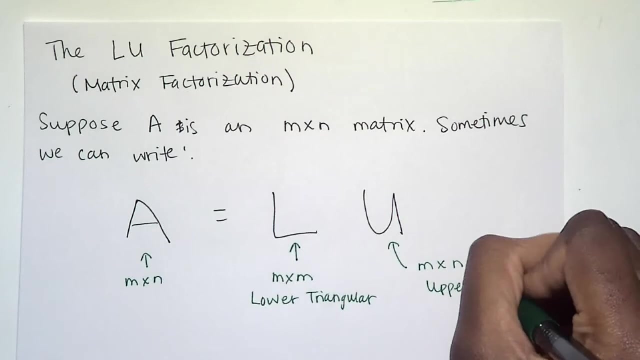 And we'll talk about what all this means. And then U is M by N and it's upper triangular. All right, so we're factoring A into these two matrix components, All right. so let's look at some examples and we'll talk about. 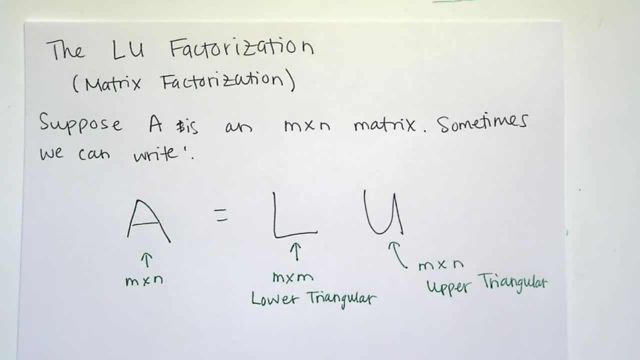 what upper and lower, upper and lower triangular means. We've seen these before, especially upper triangular. This is the same thing as our EF, So we got the zeros on the bottom. So all the stuff is on the top. Lower triangular: the zeros. 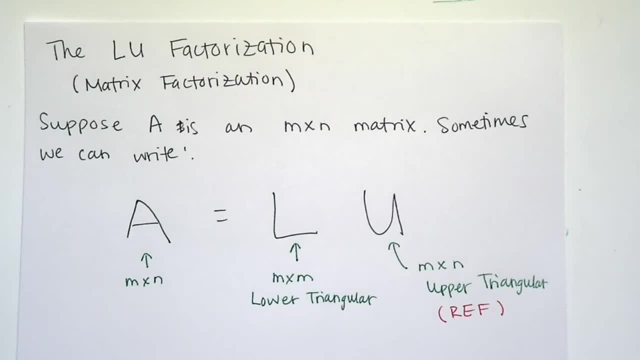 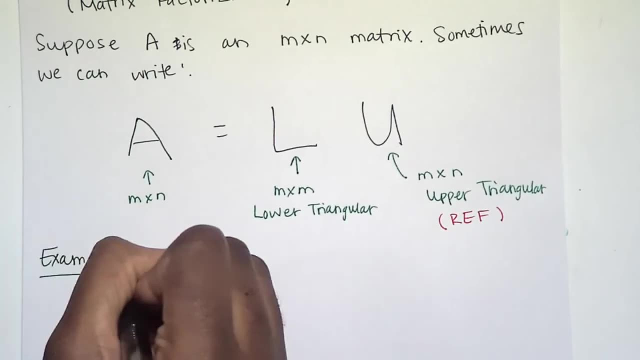 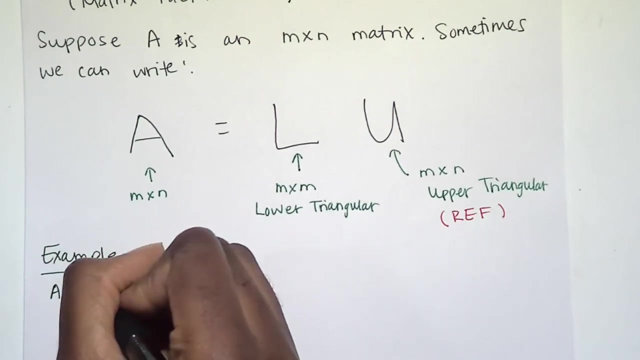 are on the top and all the stuff is on the bottom. Okay, here is our example: Matrix: A. Going down the columns, It's going to be a three by three, but just know, A can be of any type of dimension. All right, so three negative three, six Negative, seven, five. 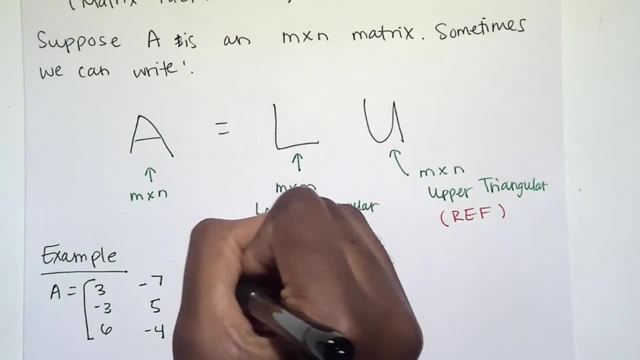 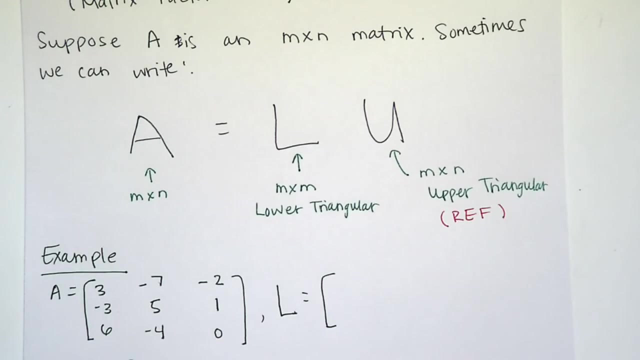 negative, four Negative two, one zero. So this is our matrix A, And it is a 3 by 3 matrix, which falls under the category of M by N. All right, then we have L. It needs to be M by M, so that means it needs to be 3 by 3.. 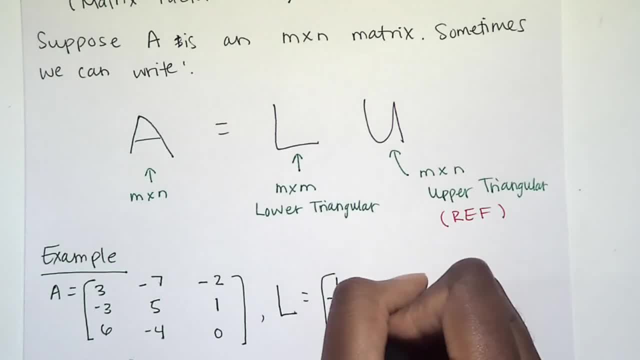 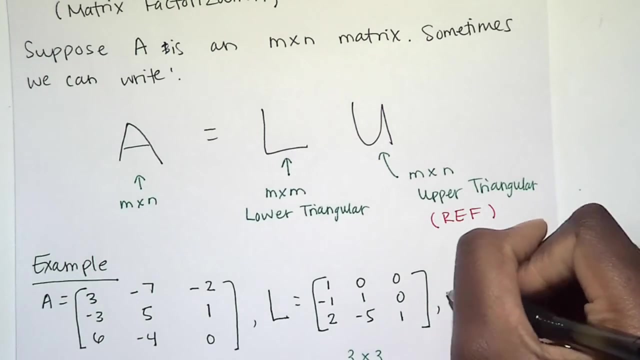 So down the columns 1, negative 1, 2, 0, 1, negative 5, and 0, 0, 1.. All right, 3 by 3.. And then, finally, we're going to have U. 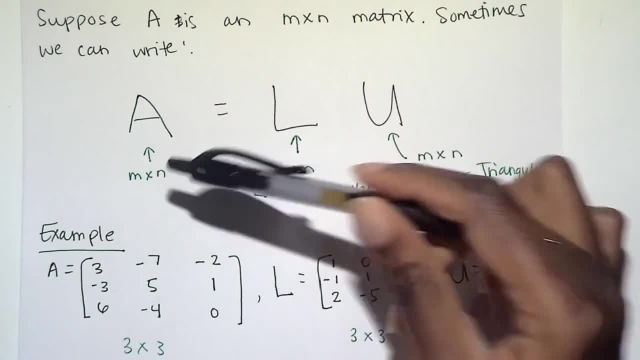 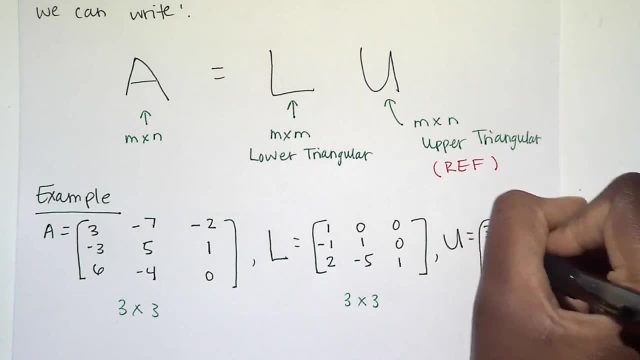 All right, this one needs to be M by N, so it needs to have the same dimensions as the original, So it should also be a 3 by 3.. 3, 0, 0, negative. 7, negative 2, 0.. 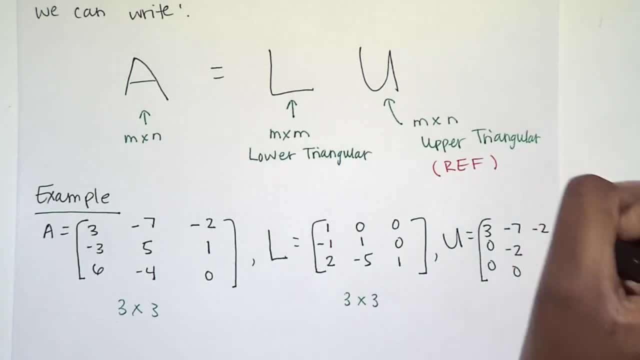 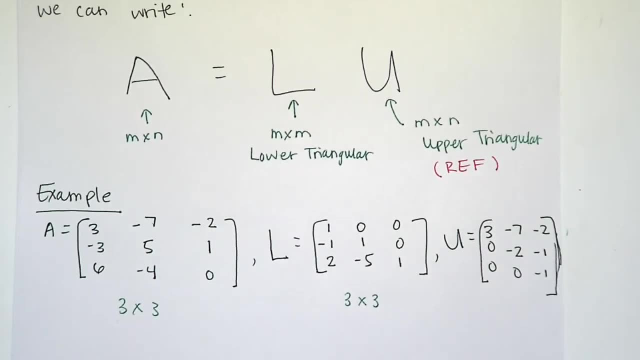 And then we have L, And then we have L- Negative 2, negative 1, negative 1.. All right, so this is also a 3 by 3.. So, it just so happens, all three of these are 3 by 3.. 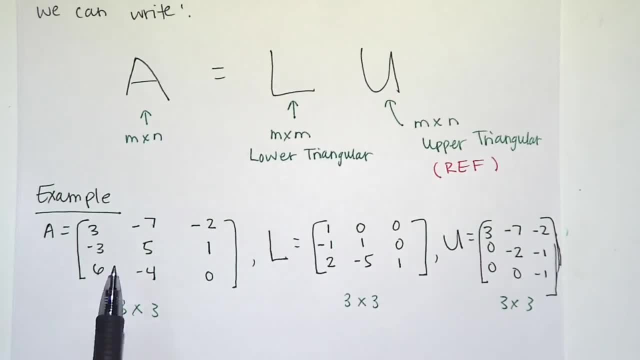 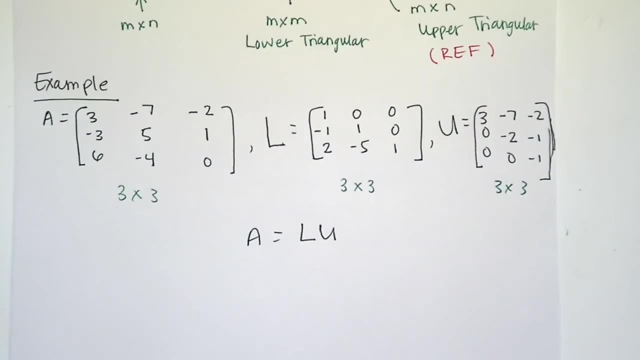 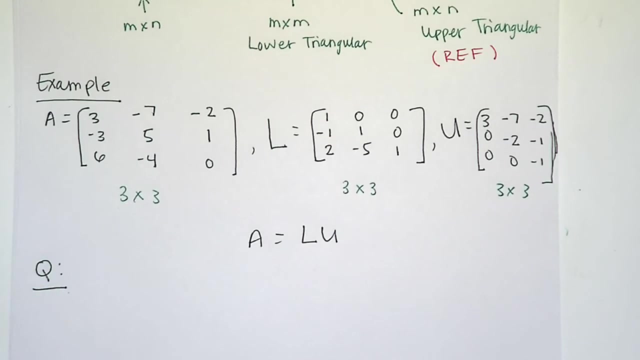 And when you multiply these two together, you'll get A All right. so why would we even want to do this? All right, let's talk. Let's talk about why It's a question. Why would we do this? Well, our goal in this class is mostly always solving linear systems. 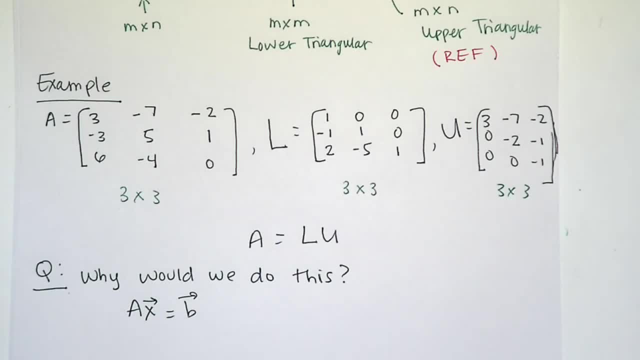 All right, so we have a system AX equals B, But according to this, we could actually do this. We could actually rewrite A as L times U. So that's what I'm going to do. So, instead of using A, I'm replacing it with L and U. 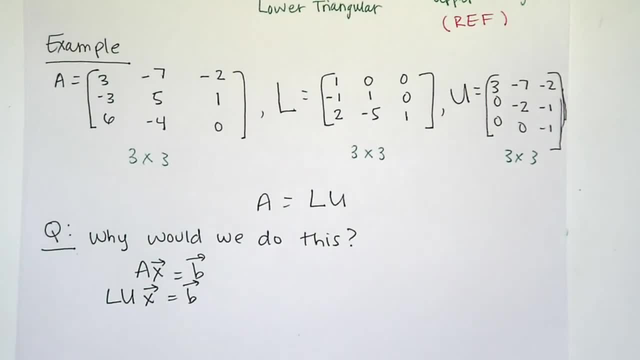 All right, now let's look at the inside here. This: U times X. This is going to be a column vector right, And I'm going to give it a name. I'm going to call this vector Y, All right, so if I replace U times X with this random letter, 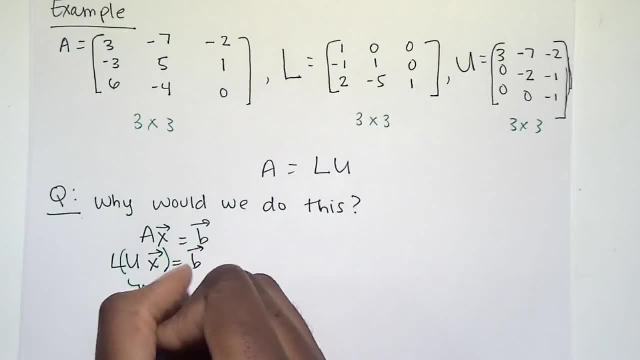 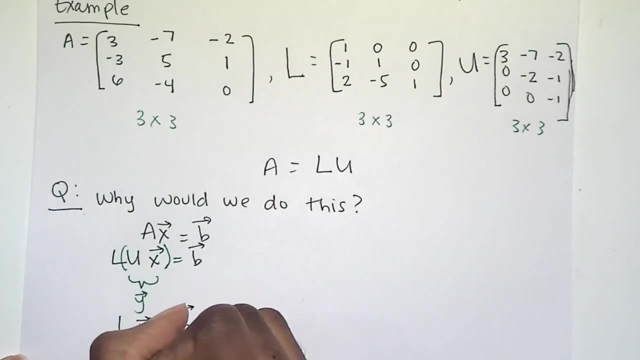 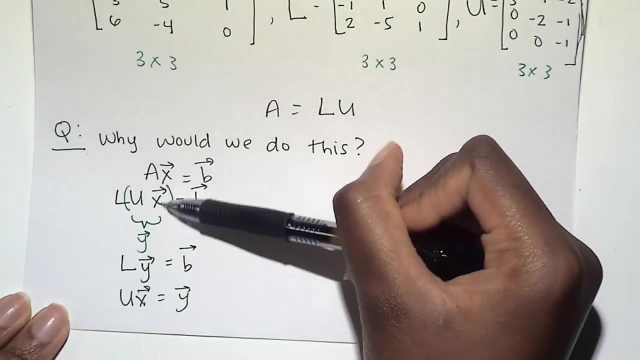 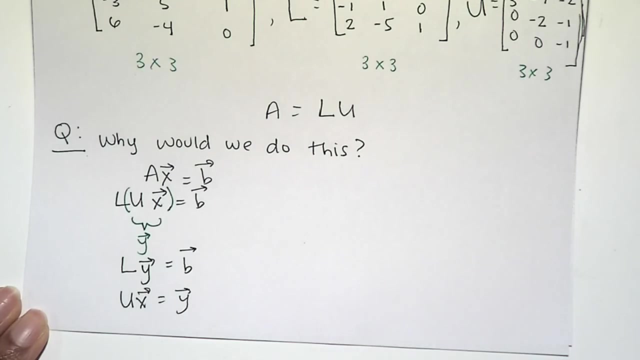 I've decided to call Y column vector. We have LY equals B, But also we need to define what Y is. We have UX. We have UX equals Y. All right, We named you X to be Y, All right. so now we actually have a pair of matrix equations to solve. 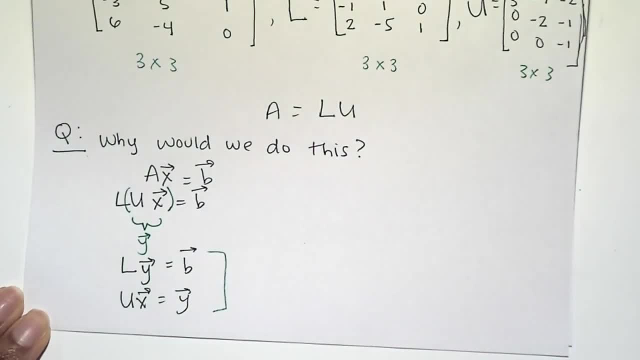 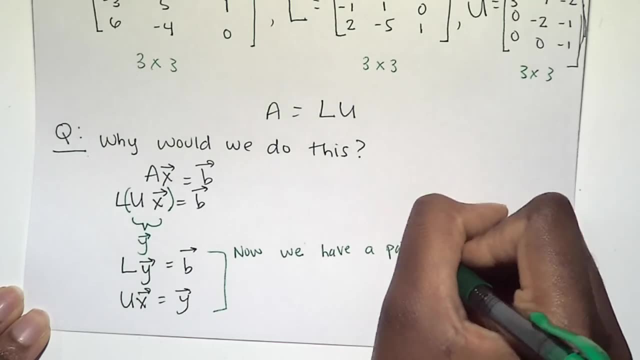 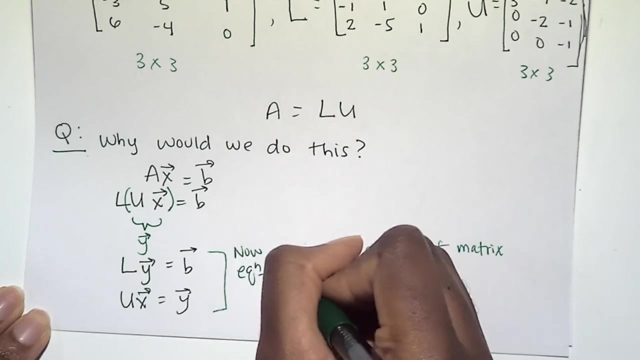 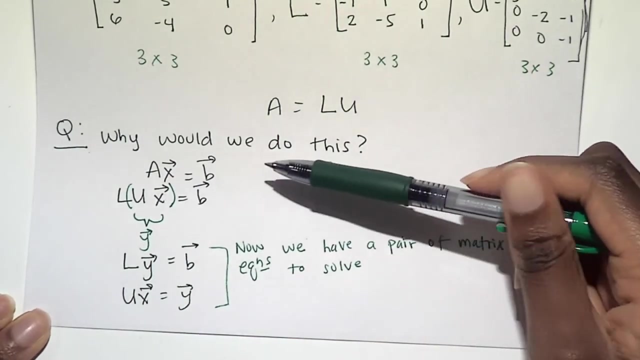 So both of these together. Now we have a pair of matrix, We have X to be Y, We have U to be Y, We have Z to be Z- equations to solve. Why would we do that? Why would we change our problem from only having one equation to?